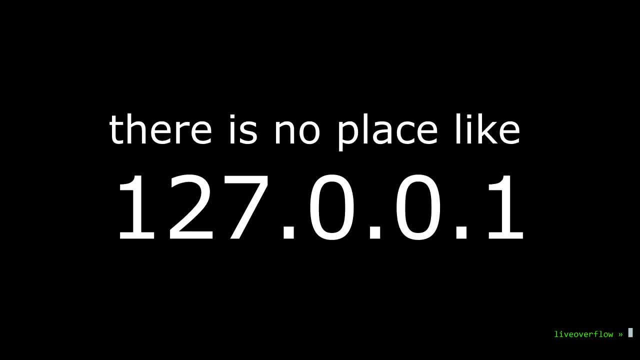 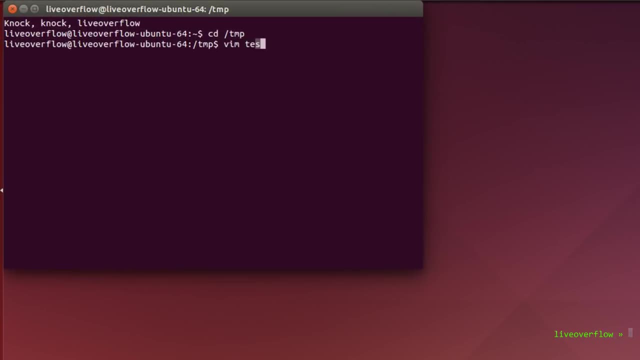 Ok, let's get started. For now we will stay on our local machine and won't make any connections to a server. We start with the displaying or rendering websites, part of the browser. So you already know that browsers can render HTML files, So let's start by constructing a simple one. 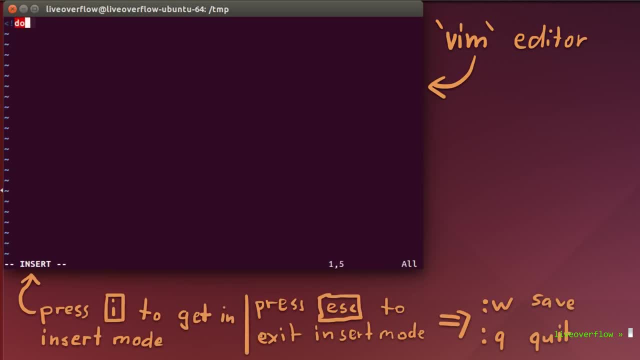 The first line is the doctype. In previous HTML versions this was more important because it included important render information for different modes for the browsers- in the past, But nowadays mostly irrelevant. Then comes the standard HTML skeleton HTML tag including a head and a body. Oh, and if it wasn't clear, HTML is hierarchical. 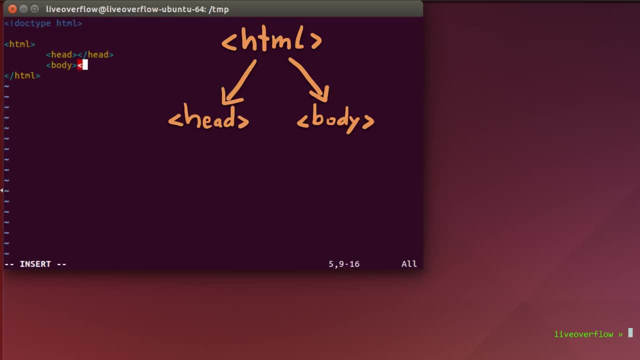 HTML tag always opens and closes again. On the inside you can have more tags, So you should read HTML always in, like the pairs of tags, and think of it in a hierarchical order. Indentation helps doing that. Let's add a heading with h1 and some text in a paragraph with p. 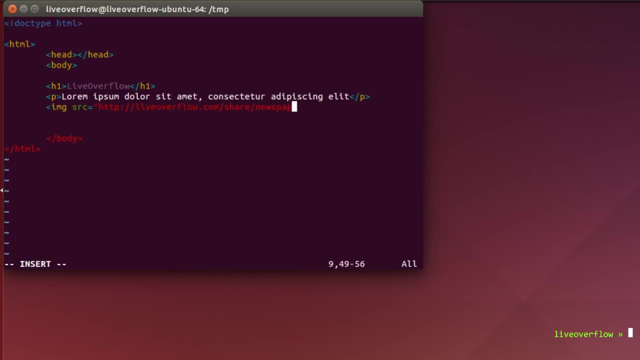 Let's also add an image with the img tag, And while we are on it, I'll link to another site. There are a lot of different HTML tags that provide different user interface features. Some are for styling text, Some are for stuff like headers or images. 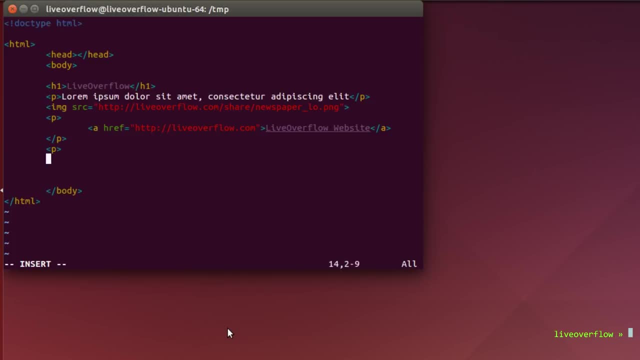 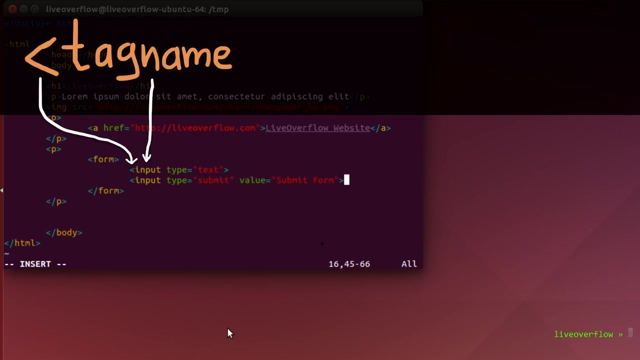 Others provide input elements for forms, So let's also add a form with a simple text box and a submit button. Generally, the syntax for tags is like this: Less than sign, followed by the tag name, without space. After that, you can have multiple key and value pairs divided by spaces. 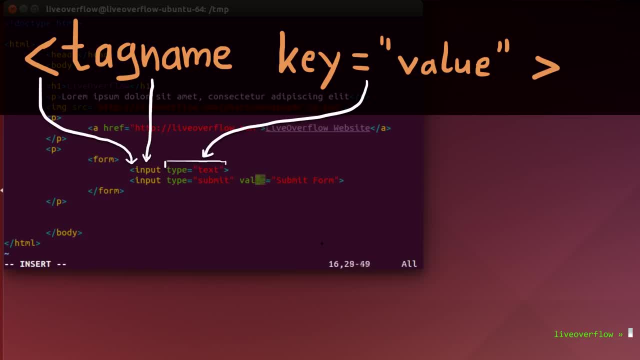 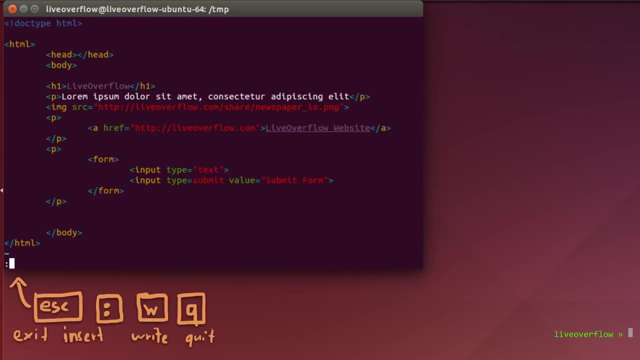 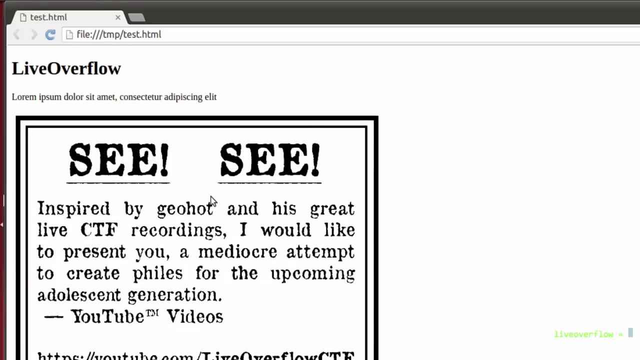 These are called the attributes of an HTML tag. The values should be quoted, but they don't have to. Another small thing that is helpful for certain attacks: Now we can open this file in the browser. The browser parses now the HTML code and starts drawing the elements to the screen. 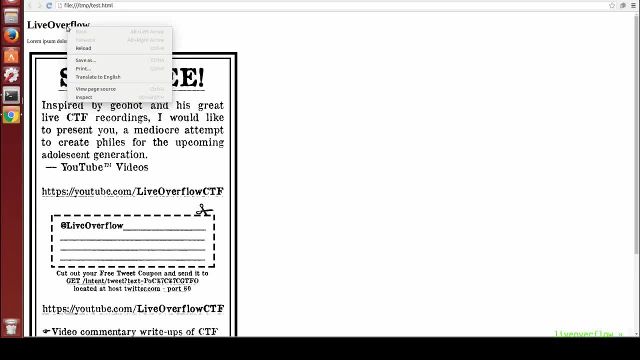 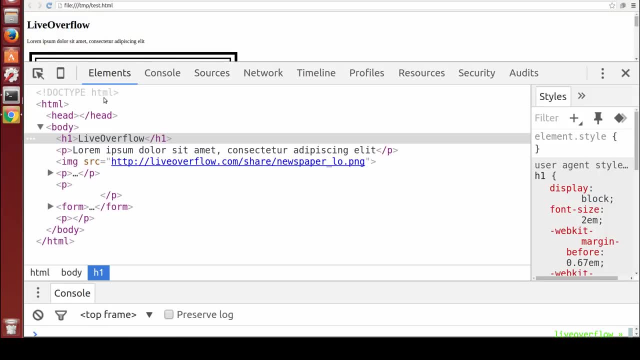 When you do a right click somewhere, you can select inspect element, which opens up the chrome developer tools. Other modern browsers have similar tools. In the first tab, called elements, you can see all the HTML document elements. This is a nice hierarchical display where you can open and collapse tags. 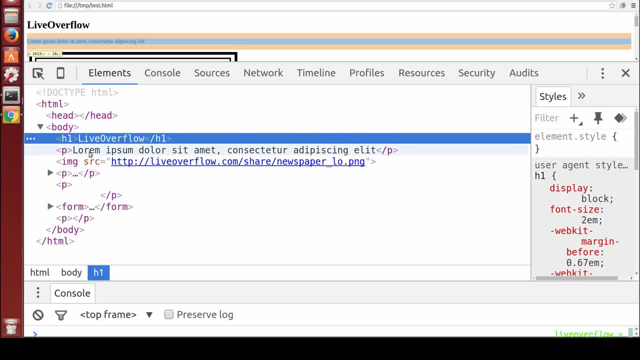 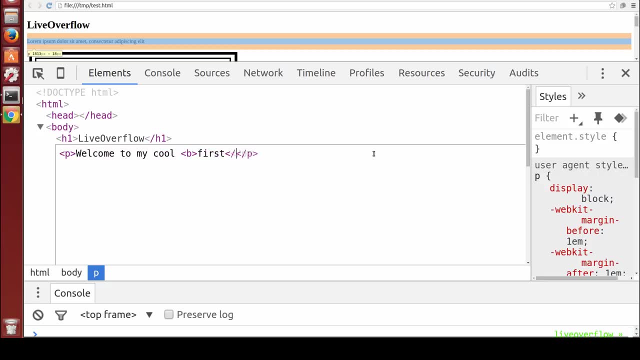 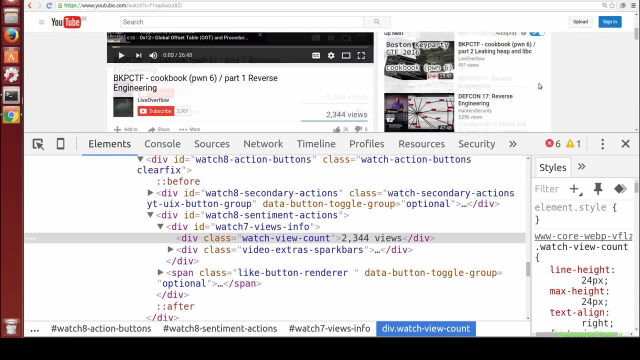 We can also go in there and change the HTML. This is obviously just changing what the browser currently displays, And when you refresh you obviously see the original file again. You are not modifying the actual file on your hard drive. Depending on your humor, that might already be enough to have fun by faking the content of a website. 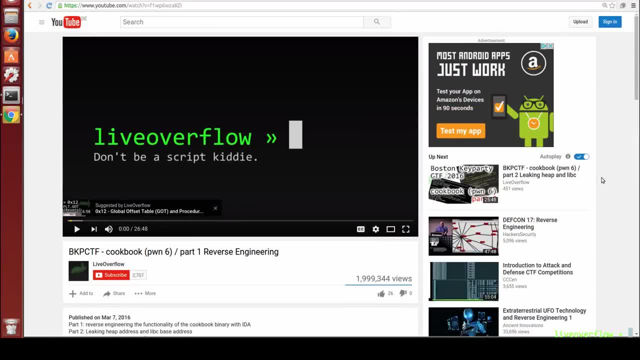 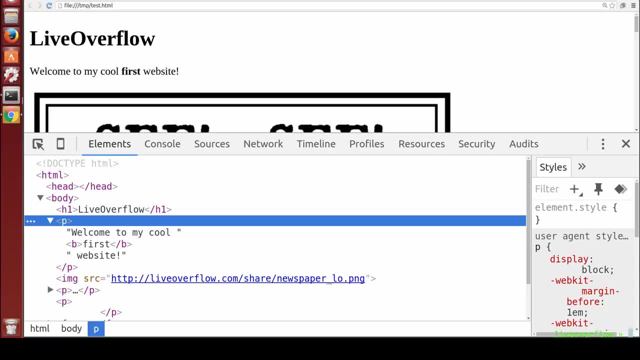 making a screenshot and post it on Facebook claiming that it was real. Browsers are also very good at something else. HTML is kinda like a programming language, But when you write some weird HTML code, the page doesn't break like a Python or C program would. 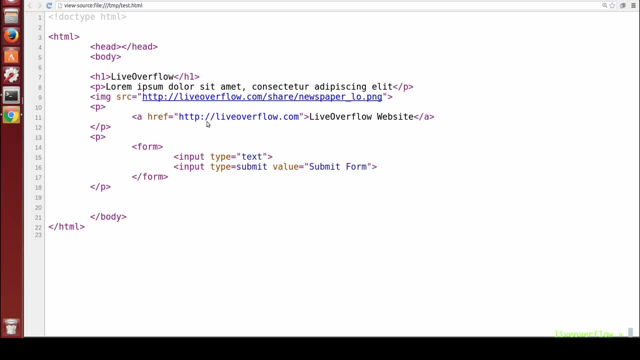 Browsers are very good at fixing crappy HTML code we write. Fixing is maybe a strong word. Let's say they are very liberal in what they accept. Here you see some examples: We put the form inside of a paragraph p tag, which is a violation of the standard. 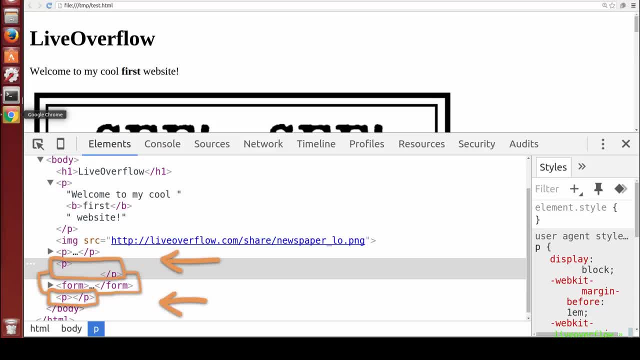 But in the inspect view you can see how the browser fixed it by making a p tag before and after the form. Other fixes include: they don't care if you forget to close your tags or they don't complain if you use weird characters in weird places. 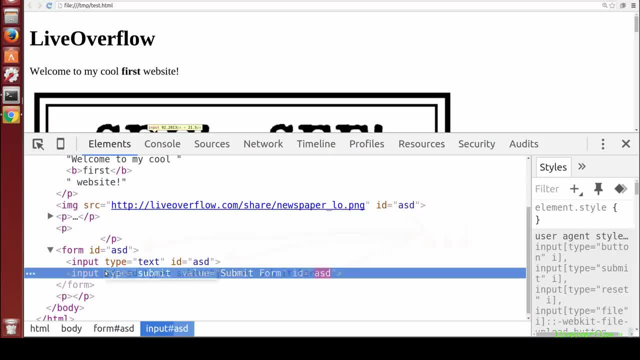 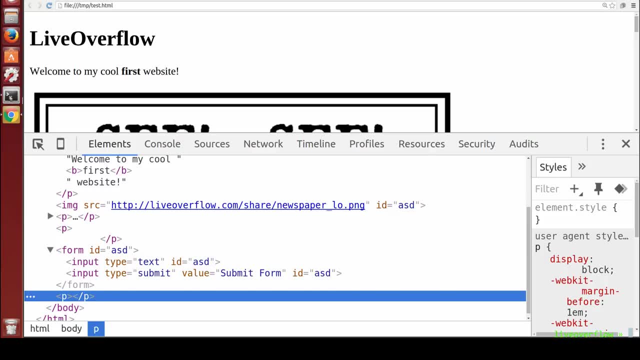 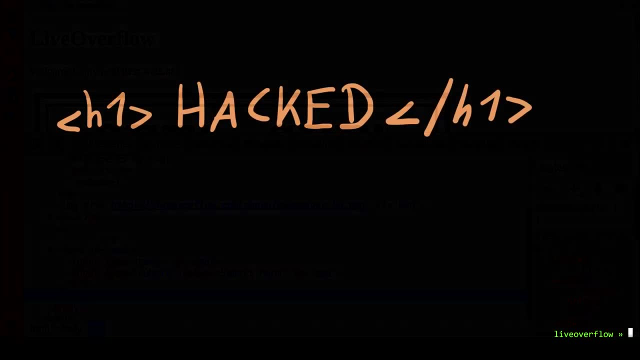 It doesn't complain about IDs that are supposed to be unique being used multiple times. You can imagine that this might add exploitation. if you are able to modify or generally inject new HTML, You can use this to get around certain restrictions, For example, if you cannot use slashes for some reason. 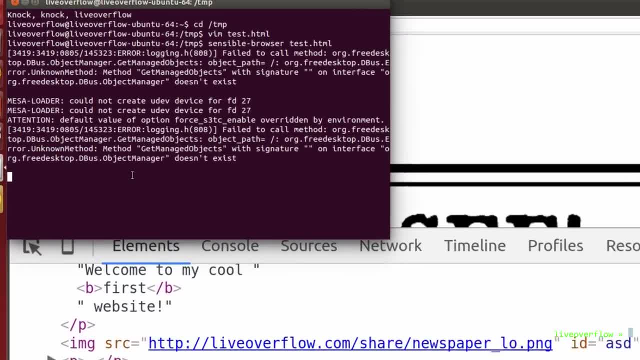 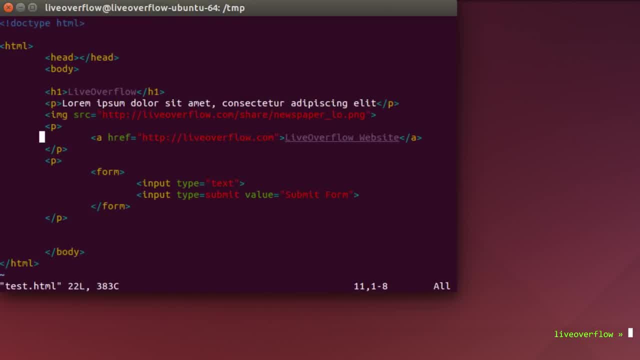 then simply don't close the tag Anyhow. besides HTML, there are a few other very common technologies used. One is CSS. CSS is another type of language that allows you to style the HTML page, For example, changing colors. You have multiple options to do that. 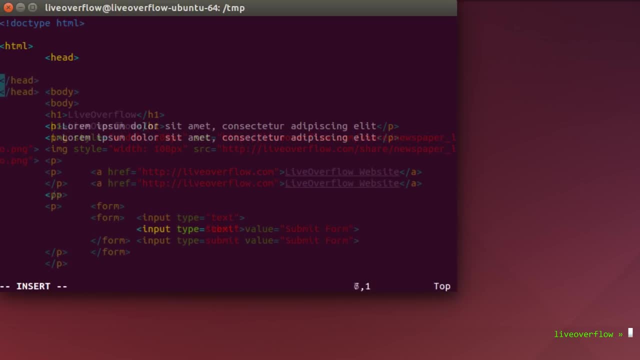 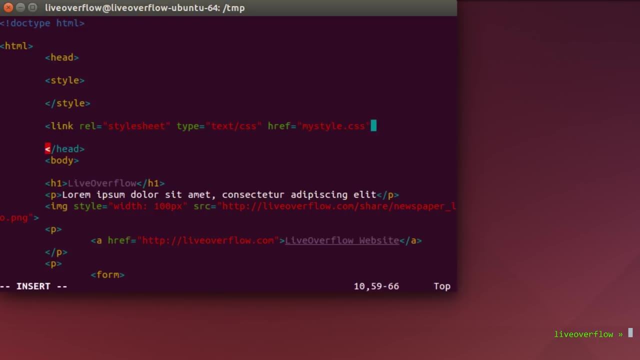 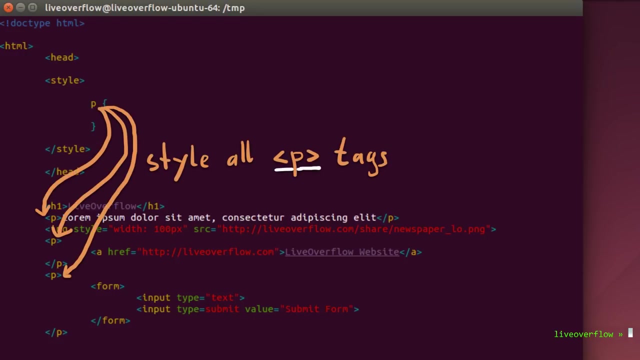 You can give each HTML element a style attribute. You can use a style tag, Or you can reference a separate CSS file. CSS syntax is super easy. You start with an identifier called the selector, So first you have to decide which HTML tags you want to style. 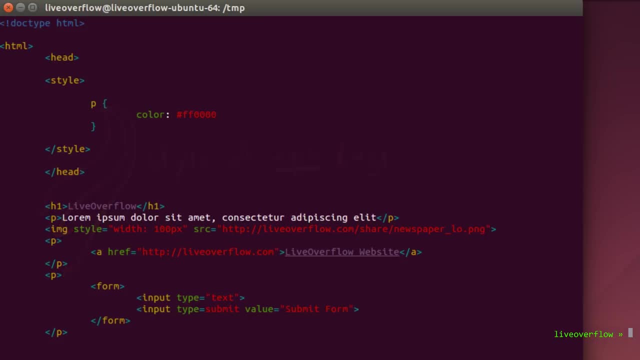 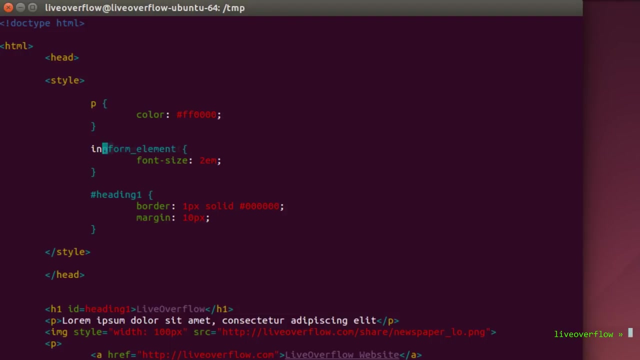 You can define styles for all tags of a certain kind Or tags with a certain class, using a dot before the class name Or only the tag with this ID, using the hash symbol. You can also combine these: Input: dot: class name references all input elements that have this class name. 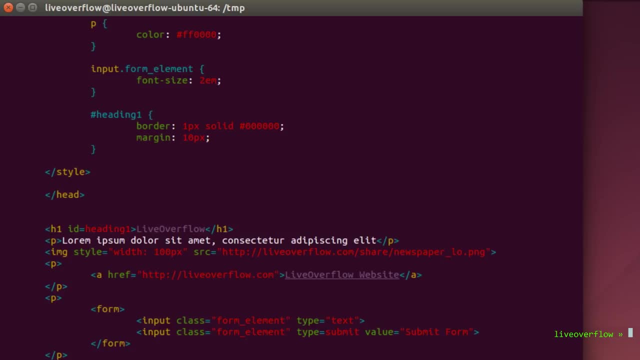 Or comma separate if you want to give different selectors the same style. Or hierarchical, only style this paragraph. if inside of something else, Inside of curly braces, you can define again key and values, This time semicolon separated. There are many different styling features. 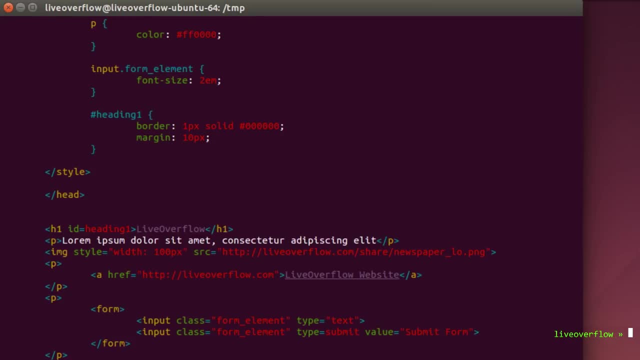 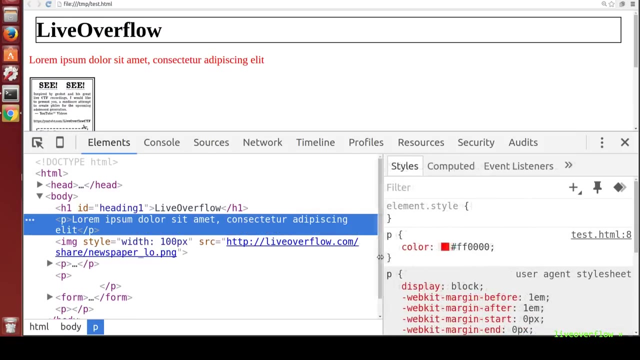 Such as text colors, fonts, margins, paddings And again. you can play with these things in the browser developer tools. Just click on an element and on the right you can make changes. It's awesome. You can immediately see the results. 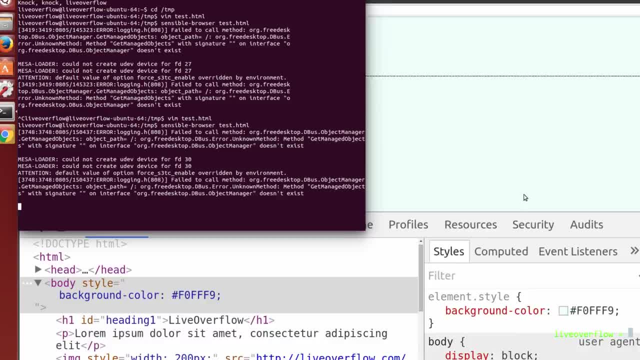 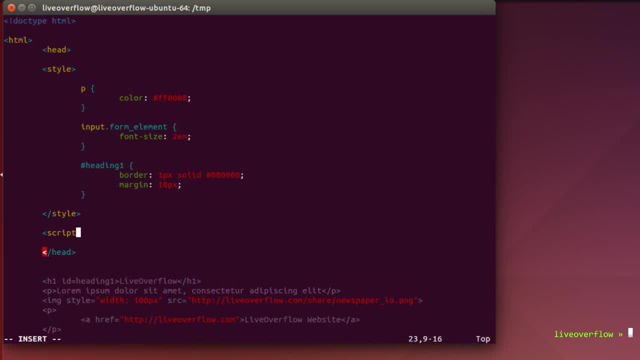 Really cool for learning. The third important technology is JavaScript. Again, you can write JavaScript inside of attributes Or use a script tag Or reference an external JavaScript file. JavaScript is a real full blown programming language, Allowing you to define functions, loops, ifs and all this kind of stuff. 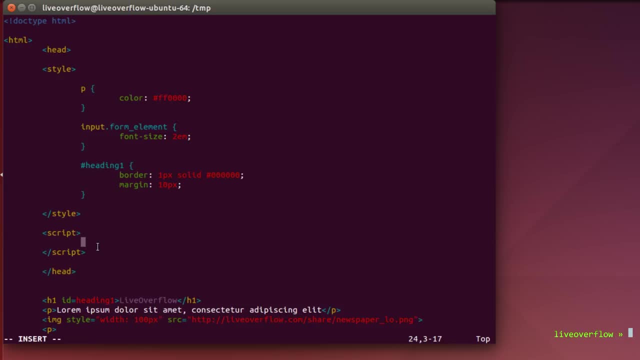 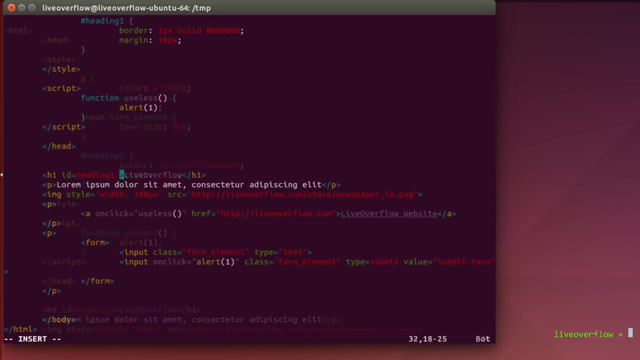 A common example and proof of JavaScript execution is to use something like alert or prompt, Which will trigger a small popup alert box. So we can, for example, define a useless function that calls alert. To have JavaScript interact with HTML, there are two different major ways. 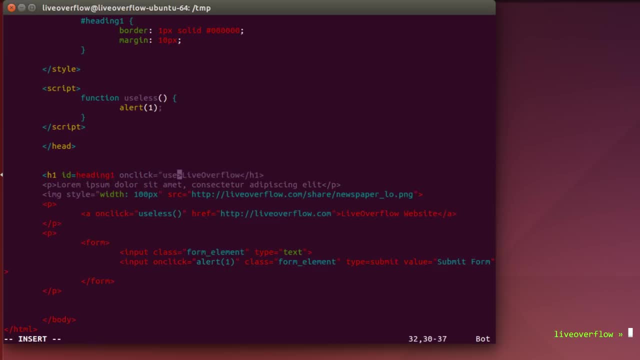 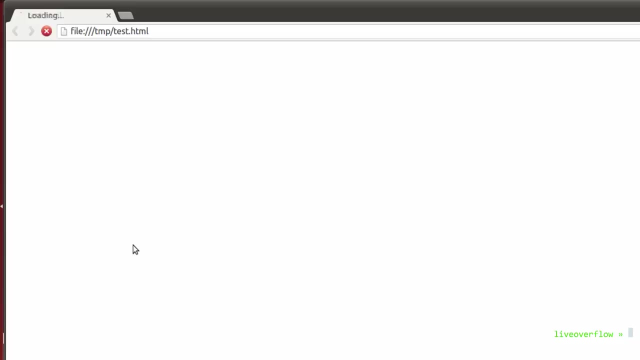 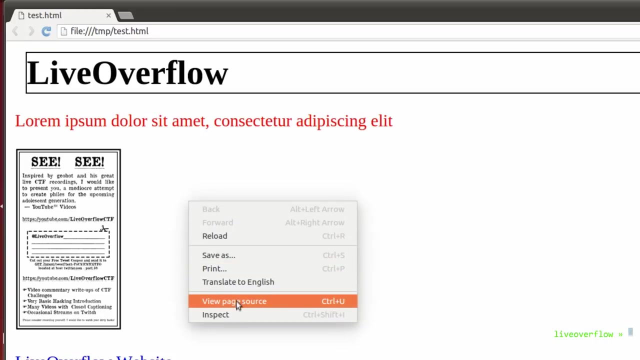 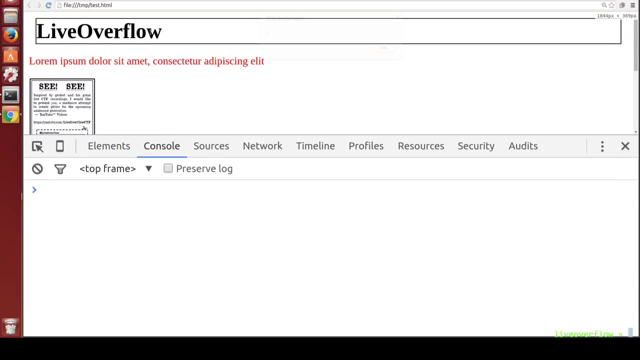 One are events. They can trigger JavaScript execution. So, for example, we can add an onclick event handler on an HTML tag And if the user clicks on that tag it will execute the JavaScript function. The other one is accessing HTML from JavaScript. You can access the HTML elements through an hierarchical object model called the DOM. 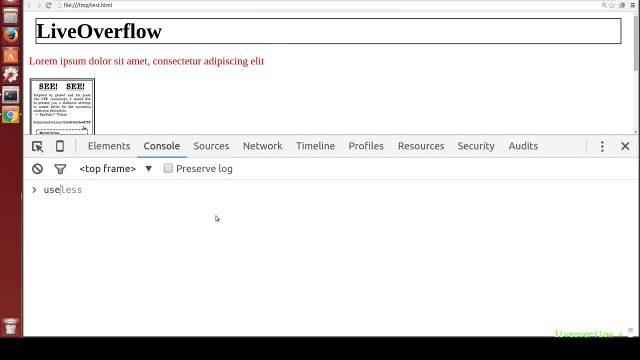 JavaScript knows objects Like other programming languages, And the DOM is simply an object representation of the HTML page So that JavaScript can exit it nicely. You can use the developer tools again to play with the JavaScript on the current site. So for example, you can take the document: